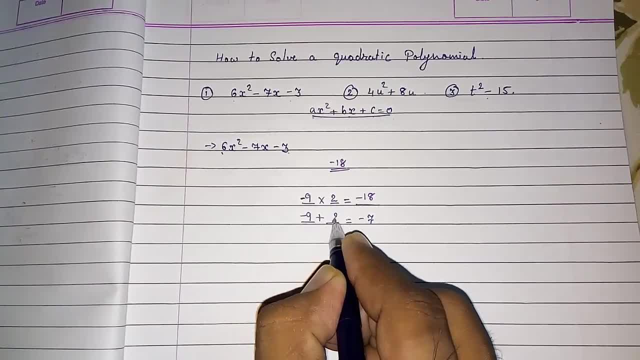 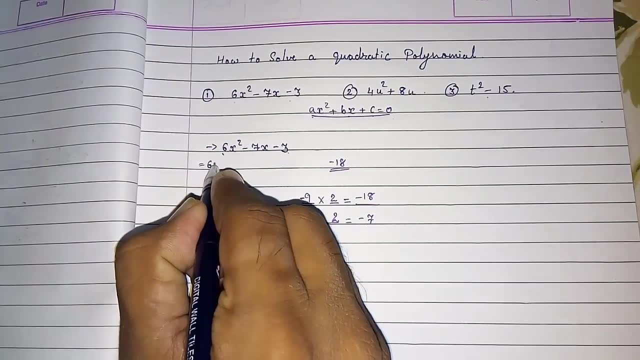 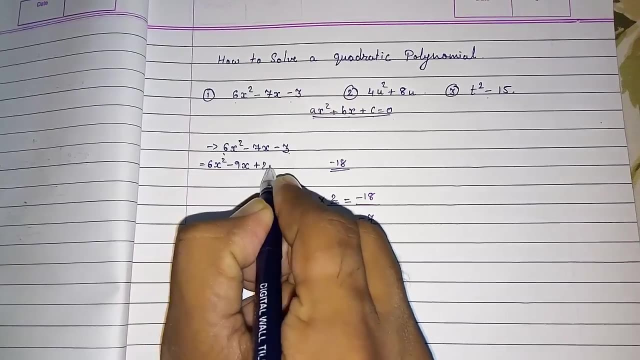 there. so we will keep minus here, because minus 9 plus 2 gives you minus 7. so your two factors are minus 9 and 2. so here we are going to solve it: x square. then we are going to split this minus 7 into two parts: minus 9, x, plus 2, x and then minus 3. now, common from this two. common from this two. 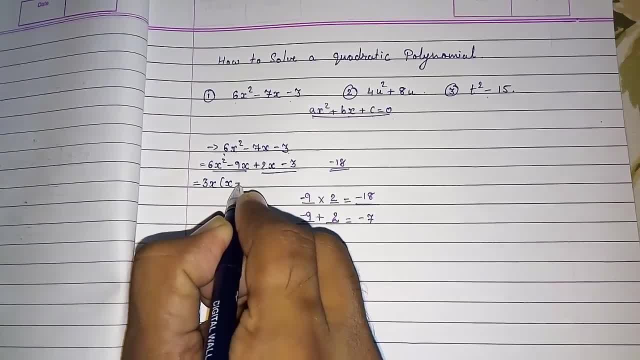 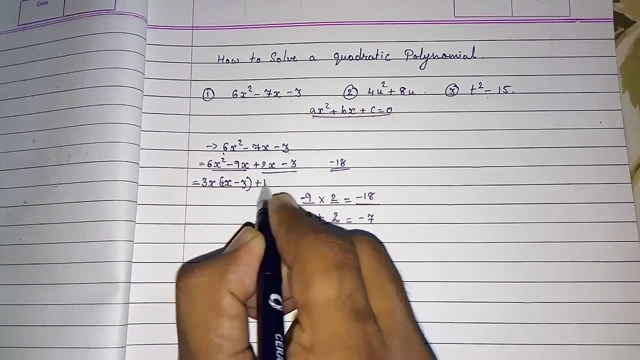 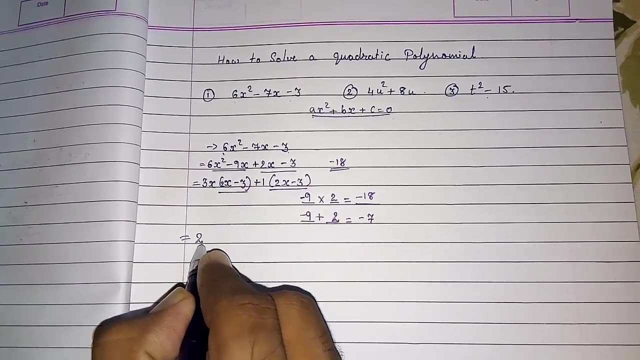 3 x will be common, x minus, sorry, 2 x minus 3, and here we are not getting anything common. so 1 and 2 x minus 3. now we are getting 2x minus 3 common in both the cases. so 2x minus 3 common and the remaining one is: 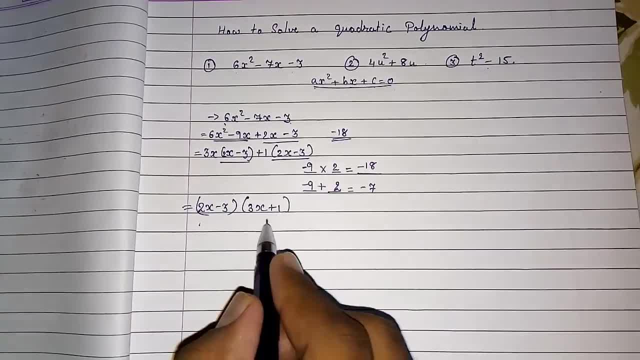 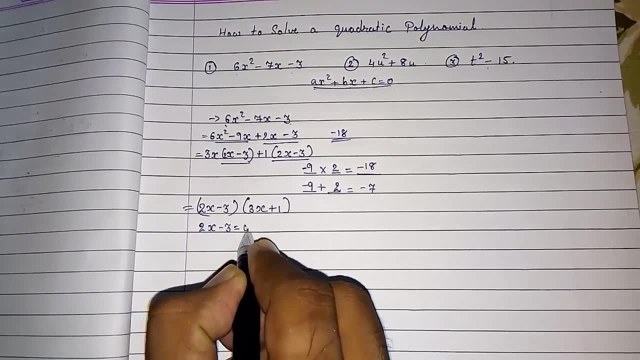 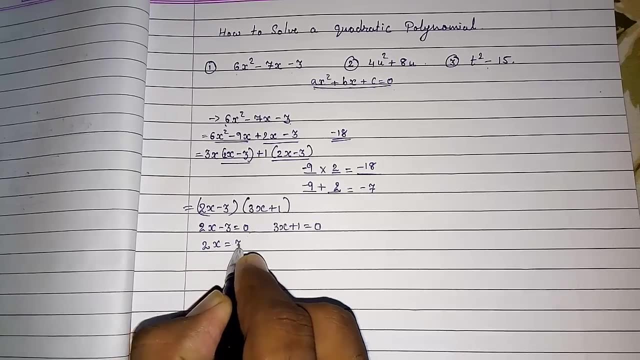 3x plus 1. so these are the two factors. these are not zeros. now we are going to find the zeros. how we can find: 2x minus 3 equals to 0 and 3x plus 1 equals to 0. now, minus v, 3 will go that side. so 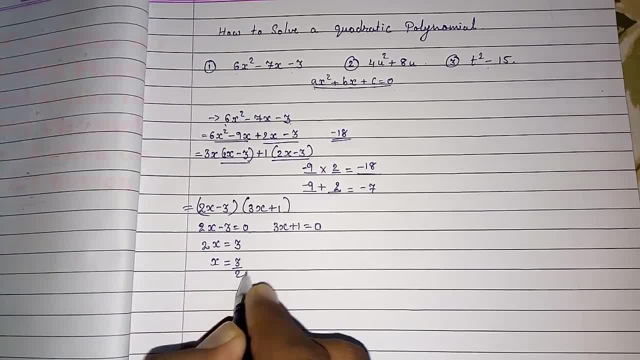 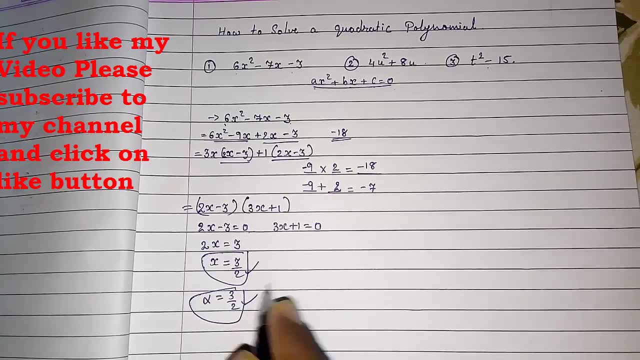 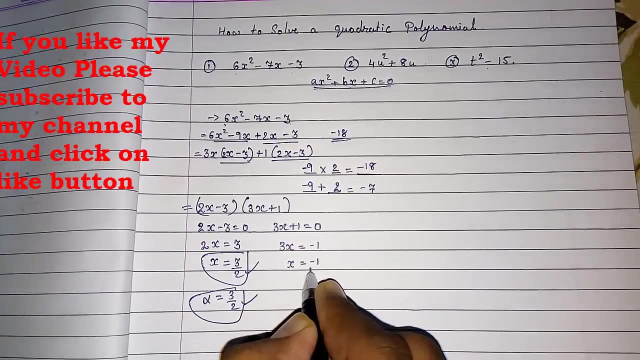 it will be plus 3, and x is equal to 3 by 2. so so this is our first 0. you can call it as alpha 3 by 2. now you will get beta from this. 3x is equal to minus 1. x is equal to minus 1 by 3. alpha- sorry. 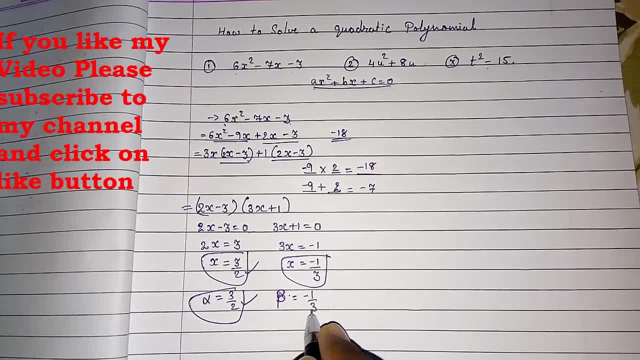 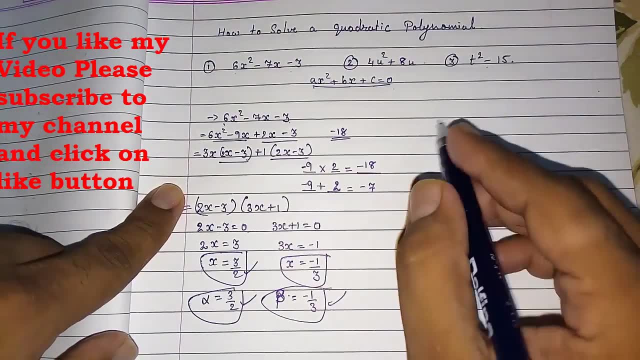 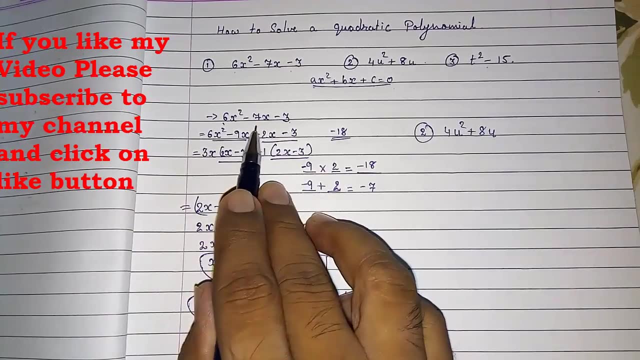 beta minus 1 by 3. these are the two zeros. it was simple, but now some changes will come in this. 4u square plus 8. in this we were splitting the middle term, but here only two terms are there. so when look here we were making four terms and 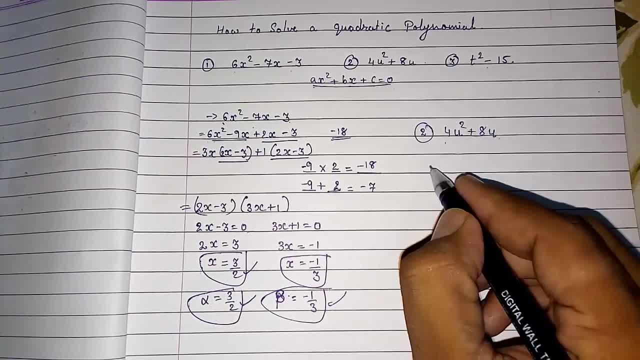 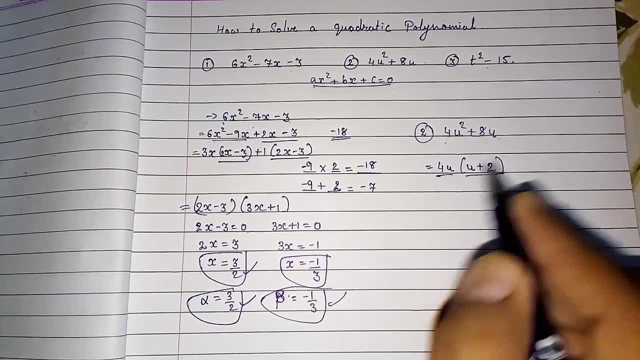 taking common from two. so here directly we will take out common as 4u and the remaining will be u plus 2. so this will be our factors and directly we can say: 4u is equal to 0, u plus 2 is equal to. 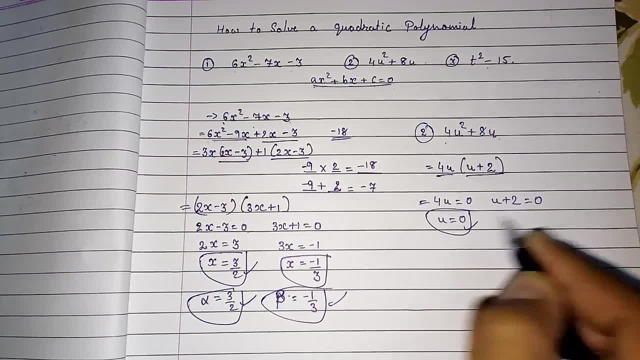 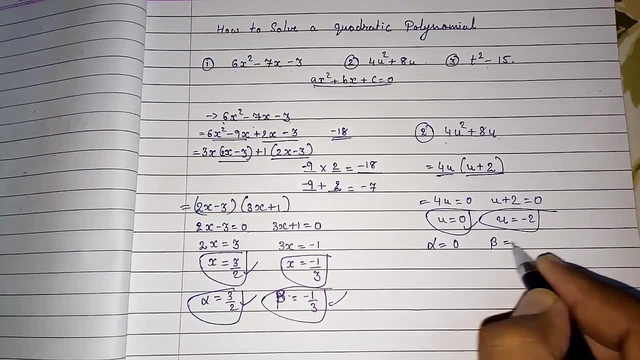 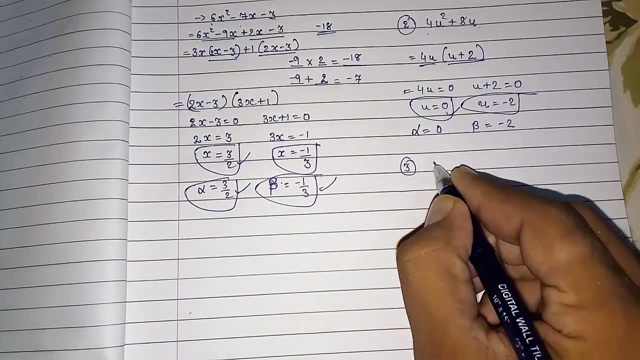 0, so u will be 0. by 4 means 0, and here u will be minus 2, so your alpha will be 0 and beta will be minus 2. now i am going to solve this third one, that is, t square minus 50. 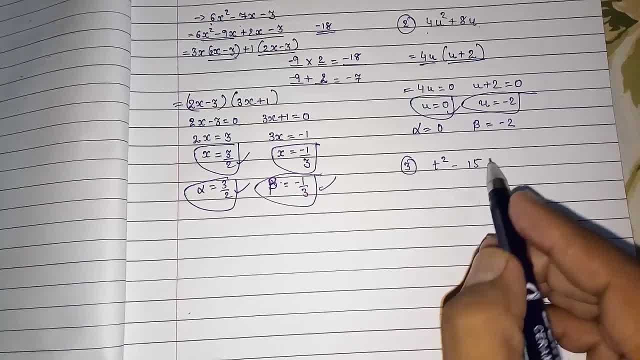 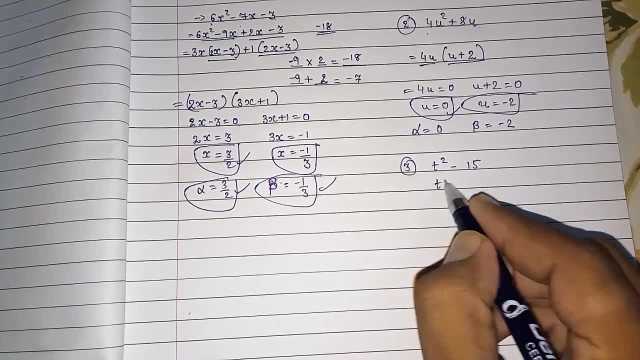 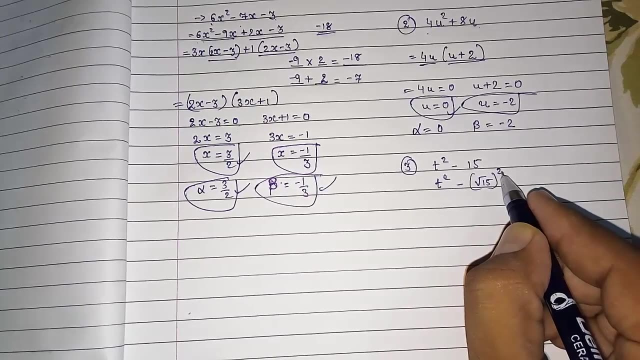 so now here, middle number is not there. so what we have to do just we have to convert this 15 into root, 15 whole square, that is t square minus root. 15 whole square means we had added root and root also and square also, so it will get cancelled and 15 will remain. but we don't want to cancel. we. 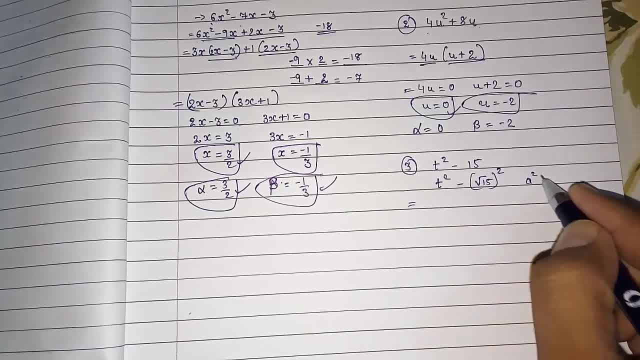 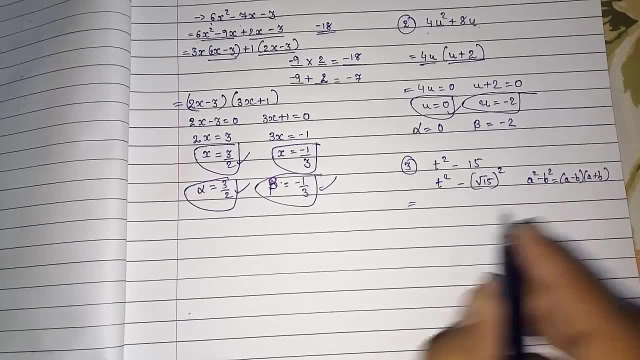 had just added, so that we will get a equation that a square minus b square identity. we know that one time it will be a minus b square identity. we know that one time it will be a minus b square identity. we know that B a plus B. so that same thing, we are going to do it here: T minus root, 15 and. 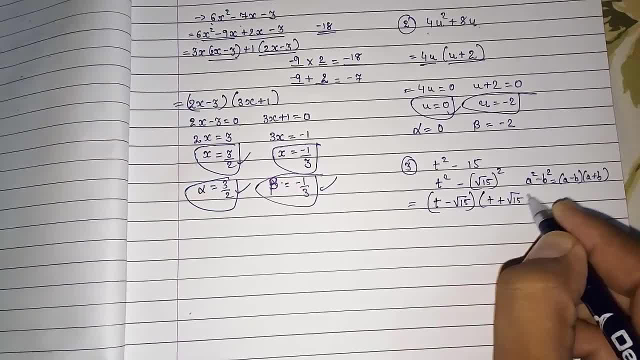 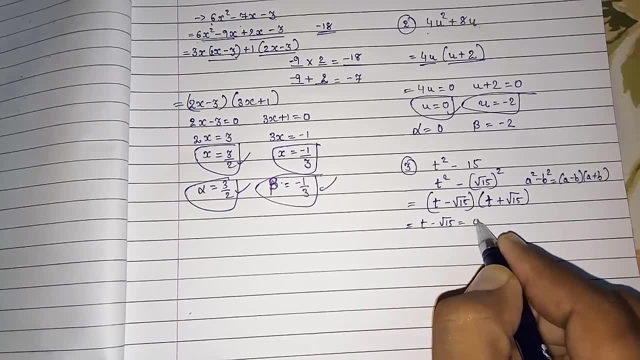 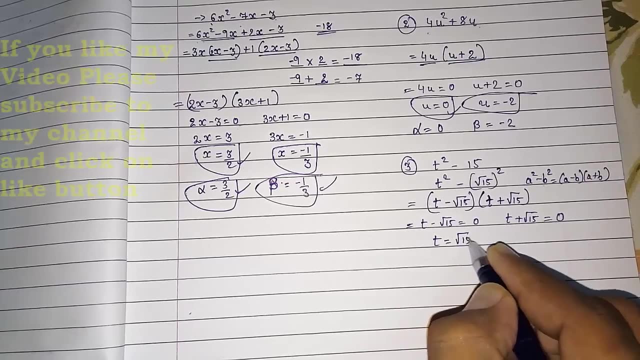 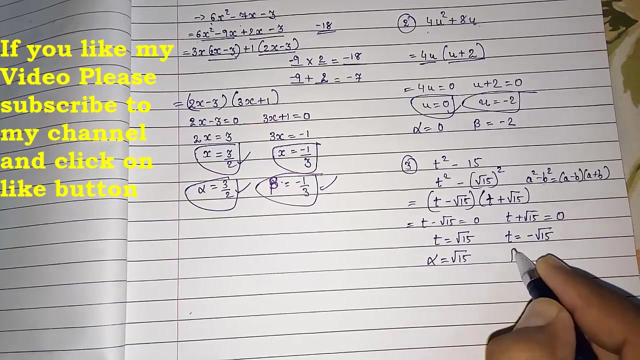 T plus root 15 will be the factors. so T minus root 15 is equal to 0 and T plus root 15 is equal to 0. so T will be root 15 and this T will be minus root 50. so your alpha here will be root 15 and beta will be minus root 50. now we 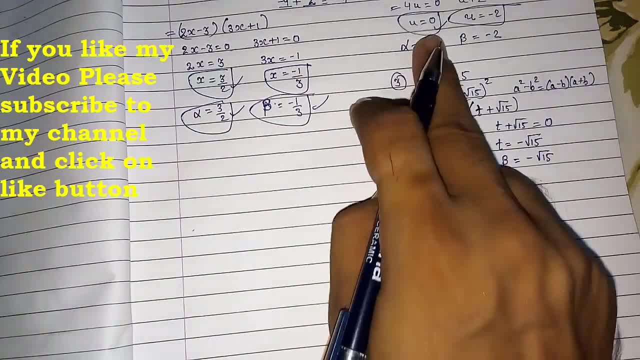 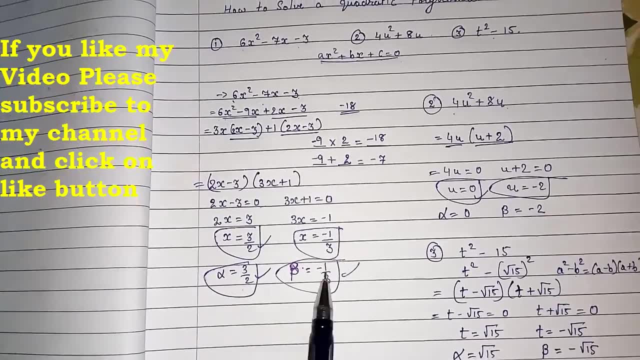 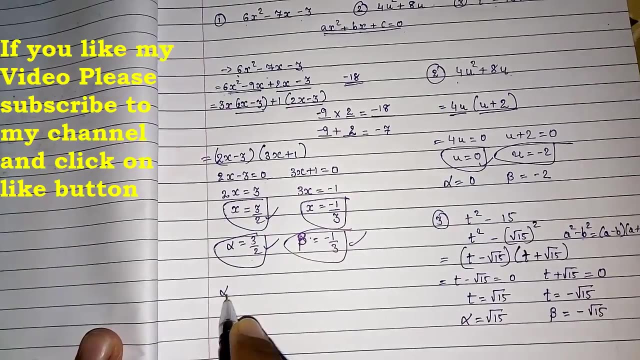 are going to verify the relationship of the zeros with the coefficient. look here here: in my first equation we had got root 3 by 2 and minus as the zeros and my question was: 6x square minus 7x minus 3. so what alpha plus beta is equal to? 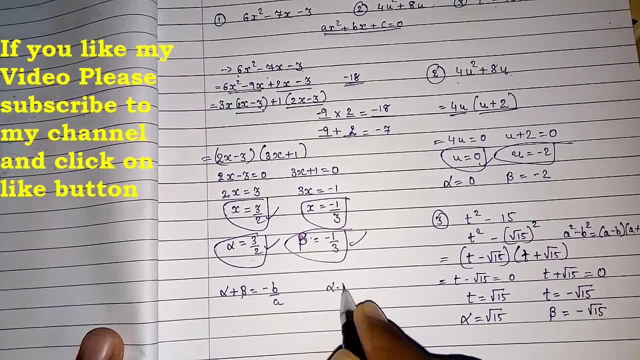 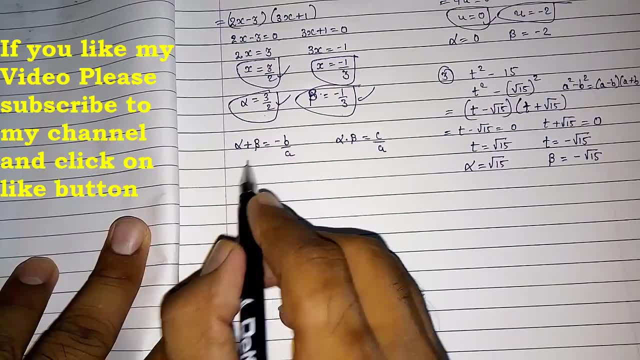 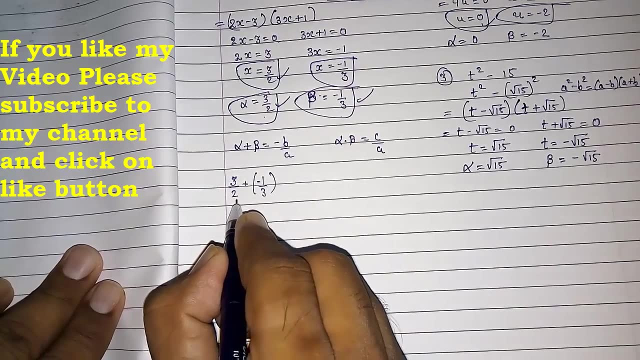 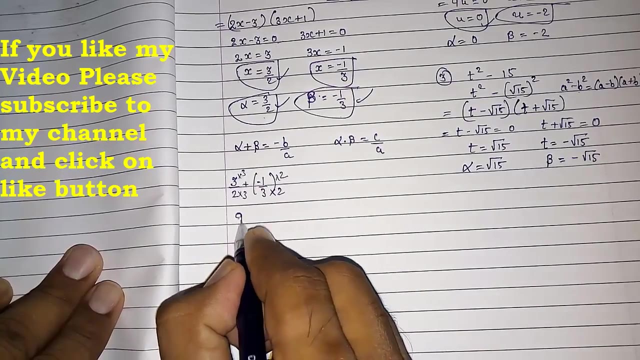 minus B upon A and alpha into beta is equal to C upon A. the answer should we will get the same answer on both the side. we are keeping 3 by 2 plus minus 1 by 3. we have to take out LCM, so here multiplying with 3 and here multiplying with 2, so we'll get 9.